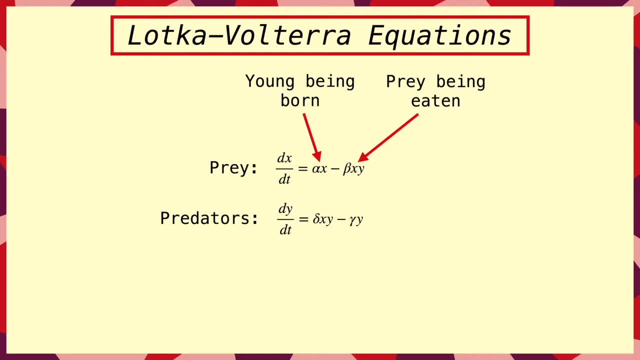 population and the predator population. This makes sense intuitively, because the more prey and predators there are, the more chances there are for them to encounter each other, resulting in a nice meal for the predator. Next for the predator, we have alphaX. 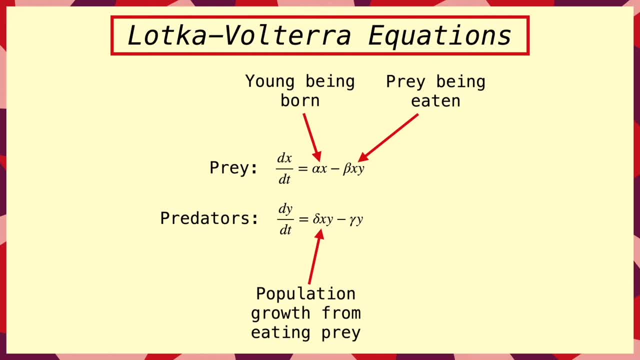 We have a term which says that the population growth is proportional to the amount of prey that they eat, and also a term to represent the natural death of the predators as they get older. Now, this is clearly a very basic model which makes lots of assumptions For. 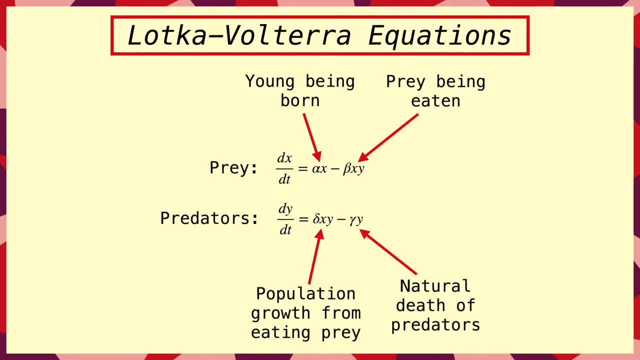 example, there's no environmental limit on the size of the populations or any limit to the appetite of the predators. So it certainly isn't perfect, but we can still look at the behaviour the system predicts and see what we can learn from it. 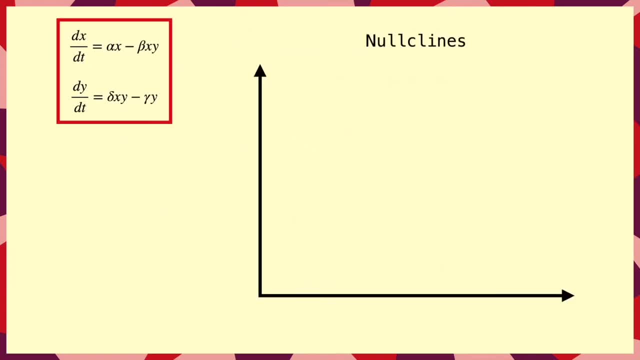 So, to analyse this system, we're going to need to construct a phase plane, which is just another way of saying a graph of X and Y which lets us see the paths that the equations predict. And whenever we do that, the first step is to find what are called NULC lines. 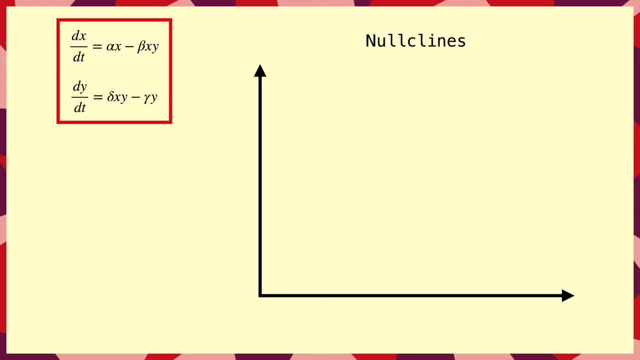 which are lines on which dx by dt or dy by dt is zero. So if we were to solve, dx by dt equals zero, Alpha X minus beta X, Y is zero And for this to be the case, either X is zero or Y equals. 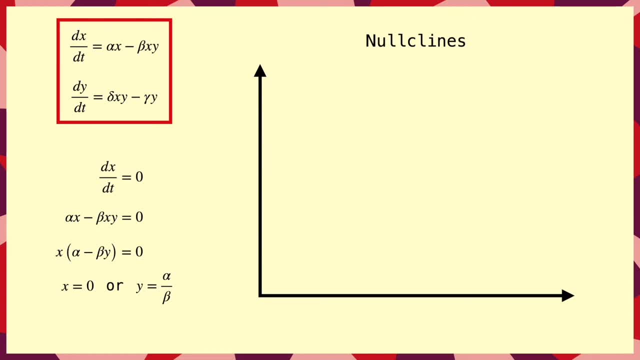 alpha over beta. And these two lines are our X NULC lines. So we can go ahead and draw these on the graph. but because dx by dt is zero on these lines, that means that only Y is changing whenever we are on these lines. so we must cross them vertically, So we'll 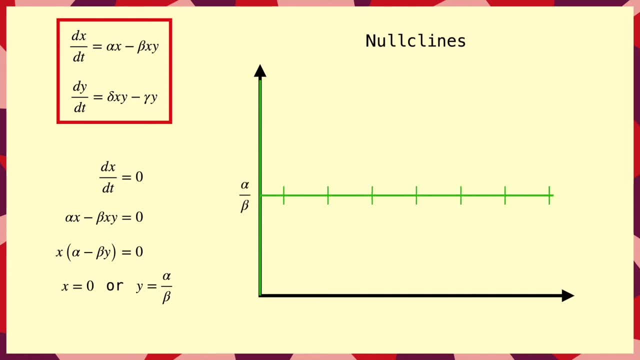 draw little ticks on them to make it clear. we need to cross them vertically. Next, we need to do the same thing for Y, so we can solve dy by: dt equals zero and we find that either Y equals zero or X is a constant gamma over delta. So we'll draw these. 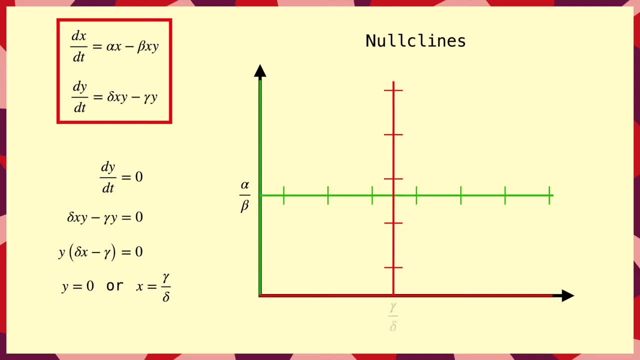 on the phase plane as well, in a different colour this time, with little ticks telling us that we need to cross these lines horizontally. Okay, so we know the X and Y NULC lines. Okay, so we know the X and Y NULC lines. Now the next step is to draw these on the graph. 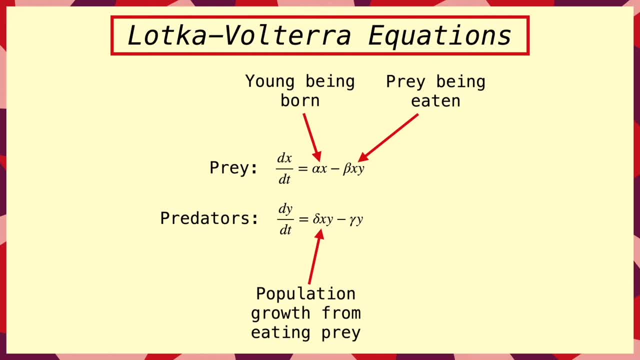 We have a term which says that the population growth is proportional to the amount of prey that they eat, and also a term to represent the natural death of the predators as they get older. Now, this is clearly a very basic model which makes lots of assumptions For. 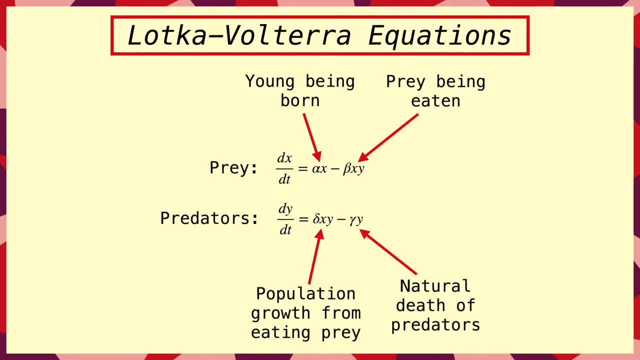 example, there's no environmental limit on the size of the populations or any limit to the appetite of the predators. So it certainly isn't perfect, but we can still look at the behaviour the system predicts and see what we can learn from it. 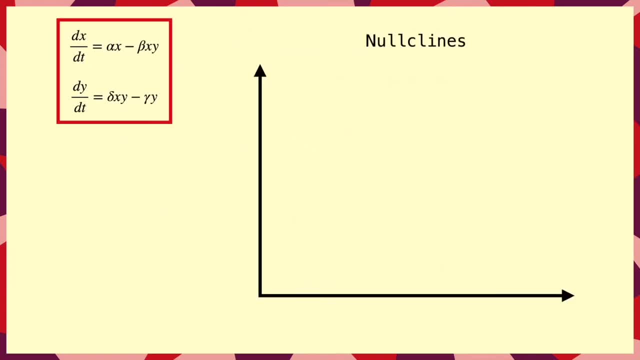 So, to analyse this system, we're going to need to construct a phase plane, which is just another way of saying a graph of X and Y which lets us see the paths that the equations predict. And whenever we do that, the first step is to find what are called NULC lines. 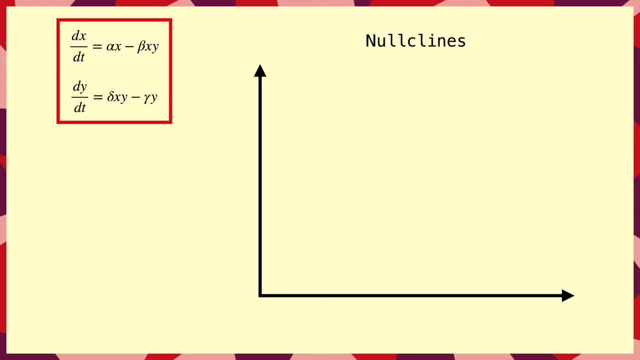 which are lines on which dx by dt or dy by dt is zero. So if we were to solve, dx by dt equals zero, Alpha X minus beta X, Y is zero And for this to be the case, either X is zero or Y equals. 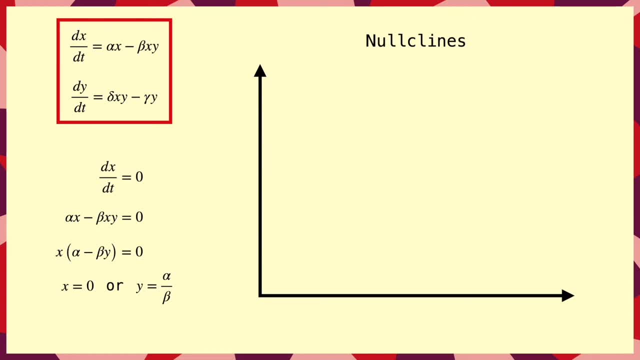 alpha over beta. And these two lines are our X NULC lines. So we can go ahead and draw these on the graph. but because dx by dt is zero on these lines, that means that only Y is changing whenever we are on these lines. so we must cross them vertically, So we'll 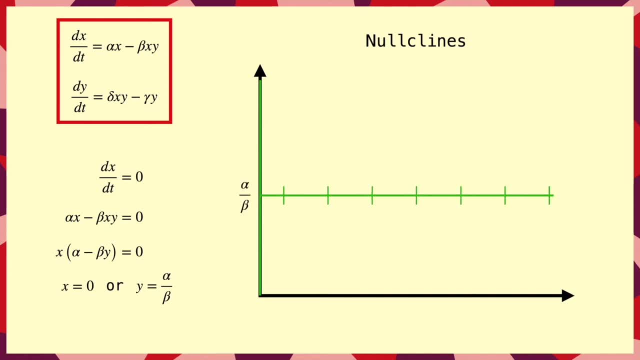 draw little ticks on them to make it clear. we need to cross them vertically. Next we need to do the same thing for Y, so we can solve dy by: dt equals zero and we find that either Y equals zero or X is a constant gamma over delta. So we'll draw. 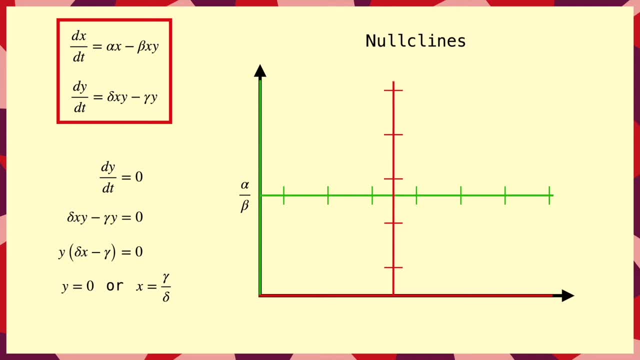 these on the phase plane as well, in a different colour this time, with little ticks telling us that we need to cross these lines horizontally. Okay, so we know the X and Y NULC lines. Now the next step is to find the stationary points, the steady states where the system doesn't. 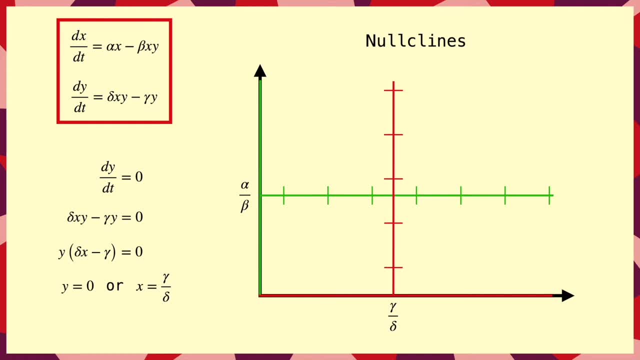 move, And these are where the two sets of NULC lines meet, And it's quite clear here that there are two fixed points, one at the origin and a second one at gamma over delta, alpha over beta. We could also have found the stationary points from the equations of: 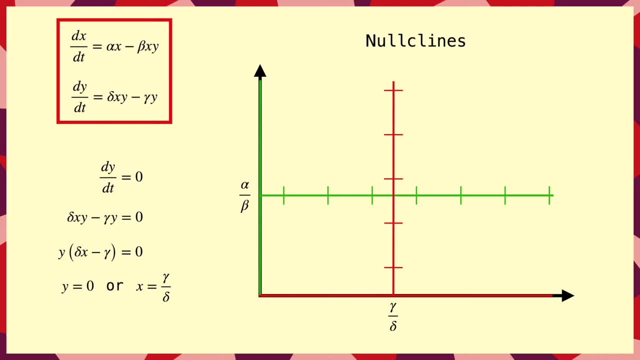 and the next step is to find the stationary points, the steady states where the system doesn't move. And these are where the two sets of NULC lines meet. And it's quite clear here that there are two fixed points, one at the origin and a second one at gamma over. 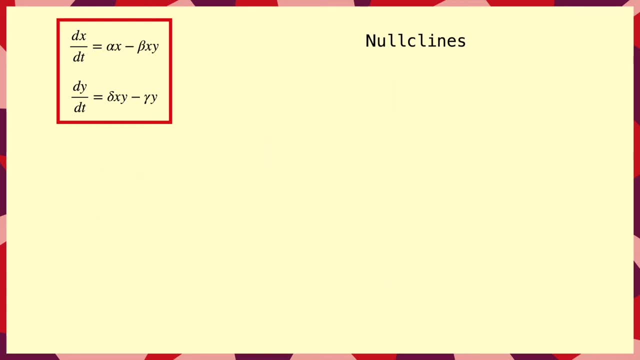 delta, alpha over beta. We could also have found the stationary points from the equations of the NULC lines. That's how you'd normally do it, but here the NULC lines are just straight lines. so it's nice, simple. So now we have our two stationary points. we want to know how the trajectories behave around. 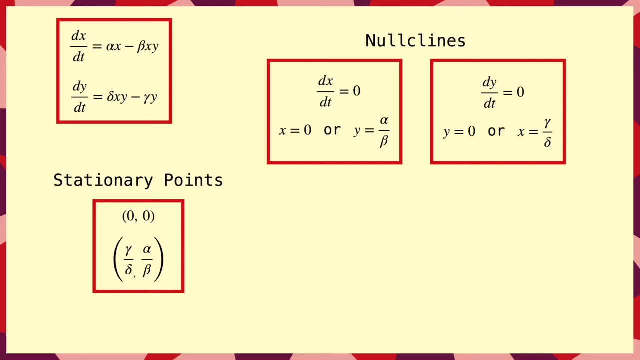 them In particular, are they stable, Do they attract trajectories towards them, Or are they unstable and the trajectories move away? Well, we can work that out by looking at the eigenvalues of this matrix M, And this just says that we take the time. derivatives of x and y. 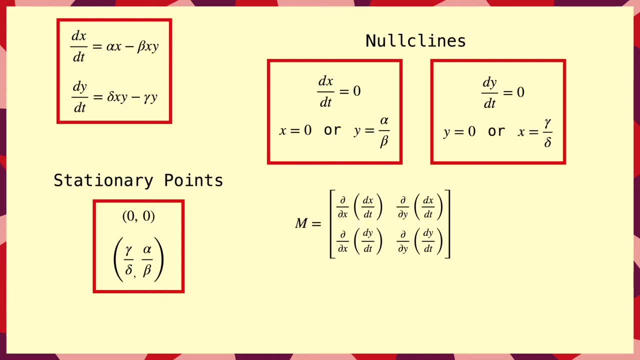 and then take the partial derivatives of those with respect to x and y and put them into a matrix. It sounds complicated and it is a little bit, but it comes from linearising the system, so taking an approximation around the stationary points to help us see whether or not they're 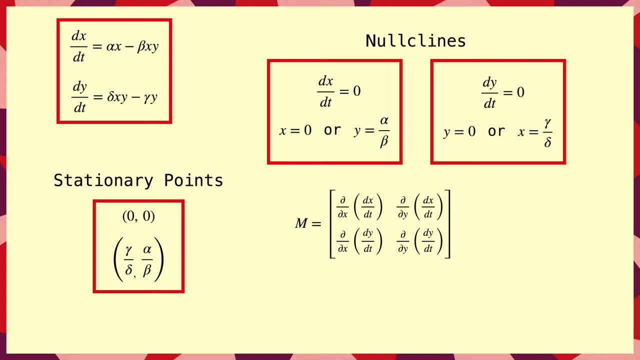 stable. I might do another video explaining the theory of where this comes from and how it works, but for now we'll just trust that it does work. So working this out. in our case, M is just this, And we'll need to evaluate it separately at each fixed point. 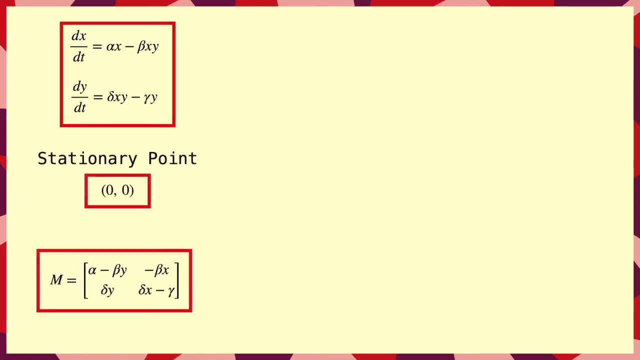 So, firstly, for the fixed point at the matrix, M is diagonal. it only has non-zero entries on its main diagonal And we can calculate its eigenvalues, although for a diagonal matrix the eigenvalues are always just the numbers on the diagonal. 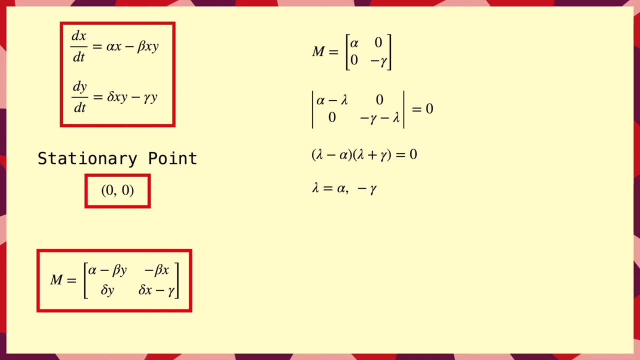 and that's what we get here. The eigenvalues are alpha and minus gamma, and since both alpha and gamma are positive, we have one positive eigenvalue and one negative one, which means this stationary point is a saddle. Now, a saddle is unstable, but we can also find the eigenvectors. 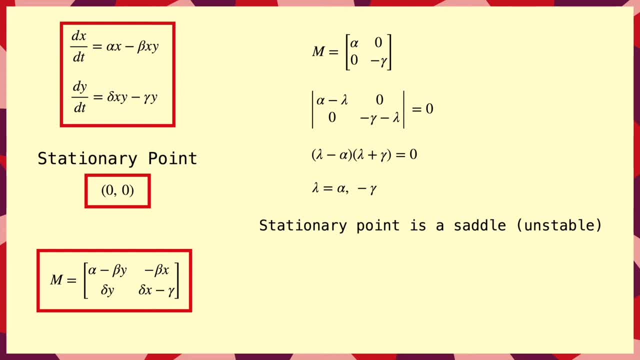 to help us see what's going on. And the positive eigenvalue, alpha, corresponds to the eigenvector in the x-direction. So this means a population of only prey grows exponentially. And the negative eigenvalue, minus gamma, corresponds to the eigenvector. 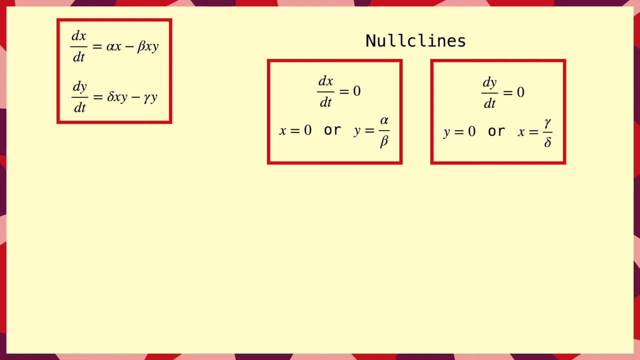 the NULC lines. That's how you'd normally do it, but here the NULC lines are just straight lines, so it's nice and simple. So now we have our two stationary points. we want to know how the trajectories behave. 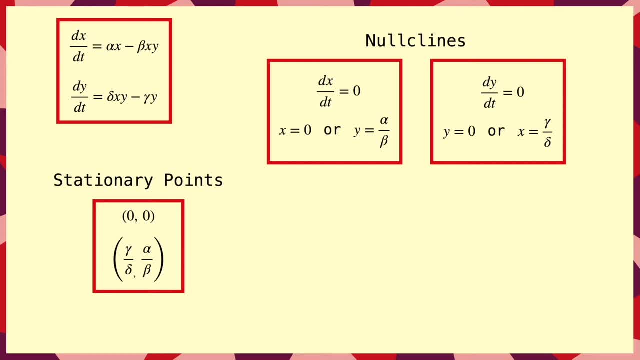 around them. In particular, are they stable, Do they attract trajectories towards them, Or are they unstable and the trajectories move away? Well, we can work that out by looking at the eigenvalues of this matrix M, And this just says that we take the time. derivatives. 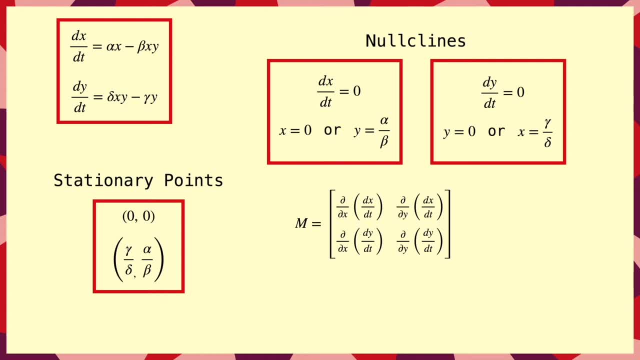 of X and Y and then take the partial derivatives of those with respect to X and Y And put them into a matrix. It sounds complicated and it is a little bit, but it comes from linearising the system. so taking an approximation around the stationary points to help us see. 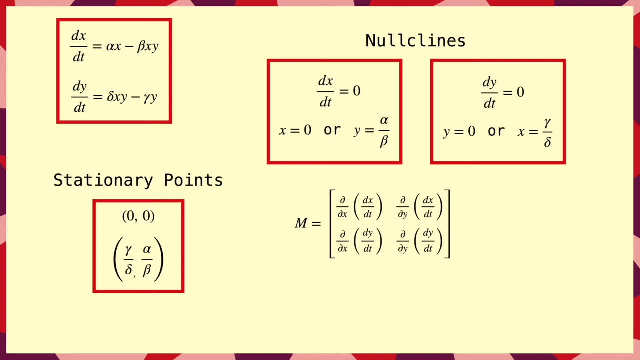 whether or not they're stable. I might do another video explaining the theory of where this comes from and how it works, but for now we'll just trust that it does work. So working this out. in our case, M is just this, And we'll need to evaluate it separately. 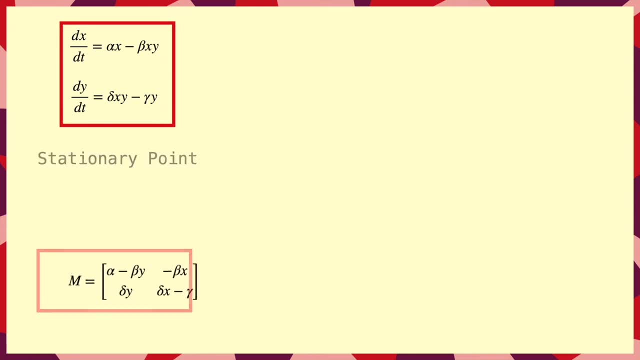 at each fixed point. So firstly, for the fixed point at the matrix M is diagonal. It only has non-zero entries on its main diagonal And we can calculate its eigenvalues, although for a diagonal matrix the eigenvalues are always just the numbers on the diagonal, and that's what we get here. 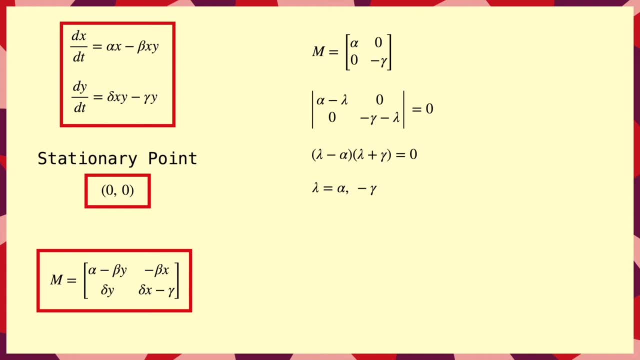 The eigenvalues are alpha and minus gamma, and since both alpha and gamma are positive, we have one positive eigenvalue and one negative, Which means this stationary point is a saddle. Now, a saddle is unstable, but we can also find the eigenvectors to help us see what's going on. 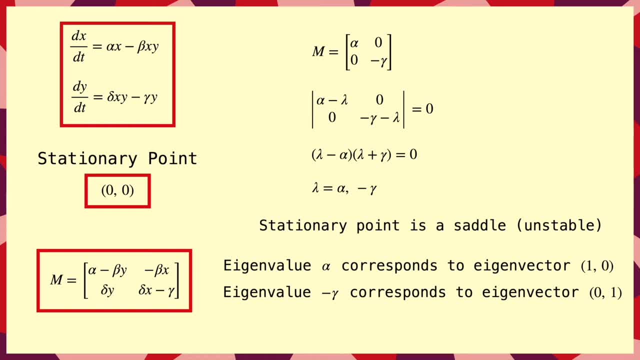 And the positive eigenvalue, alpha, corresponds to the eigenvector in the X direction. So this means a population of only prey grows exponentially. And the negative eigenvalue minus gamma corresponds to the eigenvector. And this means that if we have a population of only predators without any prey to eat, 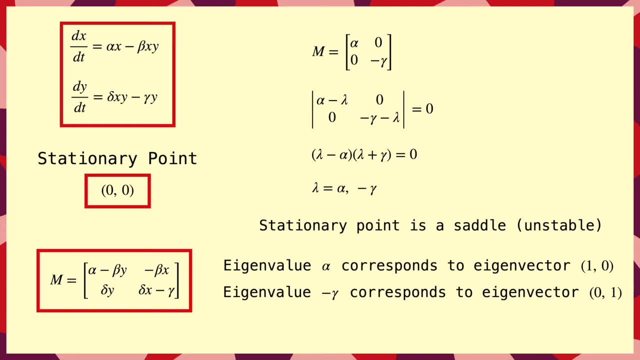 in the y-direction, And this means that if we have a population of only predators without any prey to eat, they'll die out as we expect. Next, for the non-zero stationary point, we can do the same thing, And we find that the eigenvalues 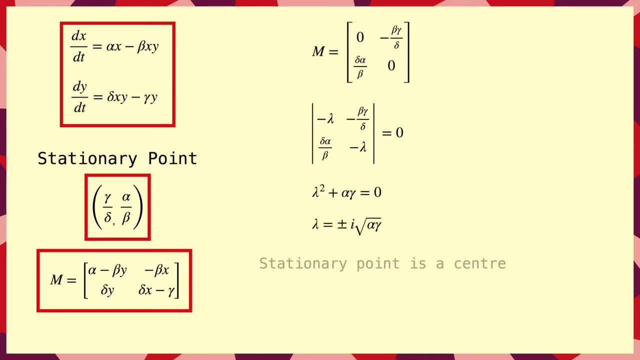 are purely imaginary, which means this point is something called a centre. It's neither stable nor unstable. Instead, the trajectories nearby look like circles or ellipses and just go round the fixed point. And now that we know about the fixed points, we can draw our phase plane. 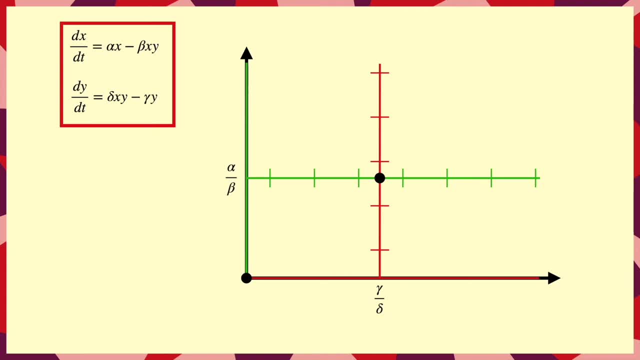 Now the nullclines split the plane into regions and we want to quickly check the direction that x and y are moving in each region. This just helps us make sure that we draw the paths correctly. So we'll put a little arrow in each region to show whether x and y are increasing or decreasing. 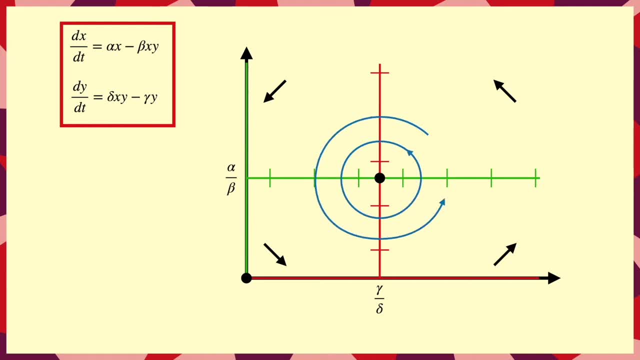 And then finally, we can draw some trajectories, making sure that the two stationary points look like a saddle and a centre. Here I've drawn the trajectories as closed loops, but we don't know that that's actually correct. They could be slowly spiralling towards. 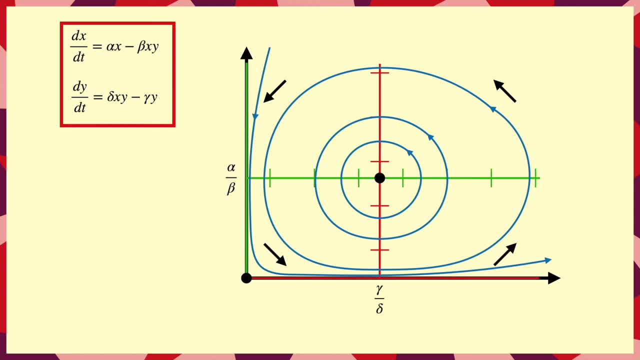 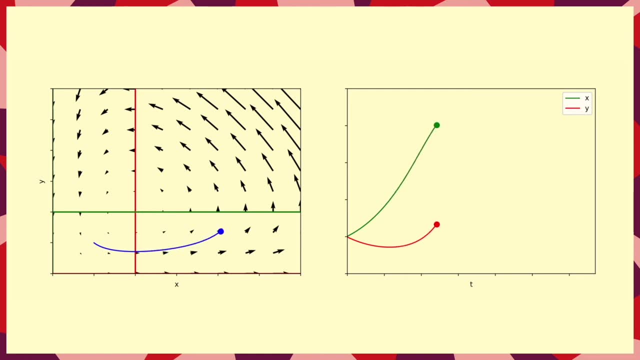 or away from the centre, But we can get a computer to draw the same thing for us. Here. on the left we have the same plot. There's a vector field in the background showing the direction and speed of trajectories, And on the right is just a graph showing how x and 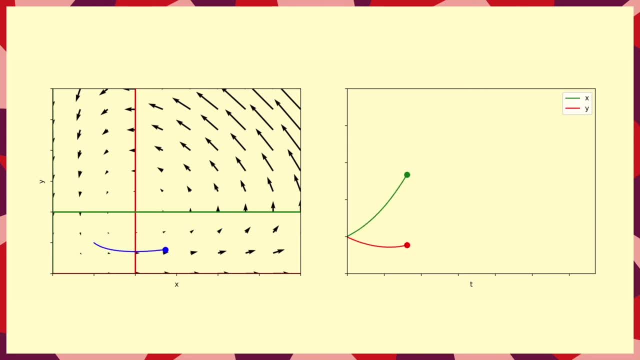 y evolve over time And we can see it looks periodic, with x, the prey population peaking first, followed by the predator population, And the trajectory does look like a closed loop. It lines up with itself each time it goes around. But can we prove why this is the case? Well, if we. 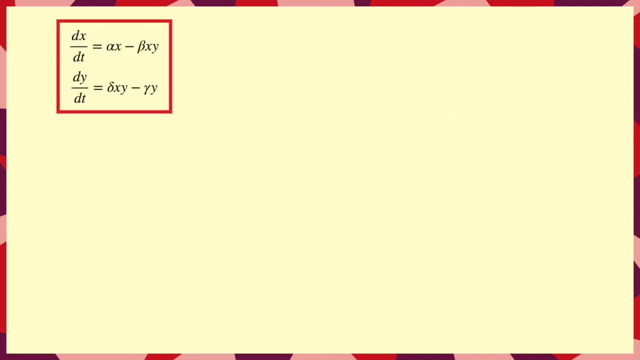 want to do that… to look for a conserved quantity, a bit like energy in a physical system. So we need to find some combination of variables whose time derivative is zero. Well, to begin with we can multiply our equations by delta and beta so that the xy terms cancel out. but then 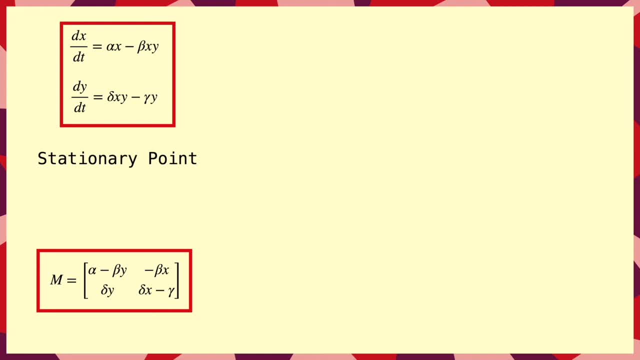 they'll die out, as we expect. Next, for the non-zero stationary point, we can do the same thing, And we find that the eigenvalues are purely imaginary, which means this point is something called a centre. It's neither stable nor unstable. Instead, the trajectories nearby look like circles or 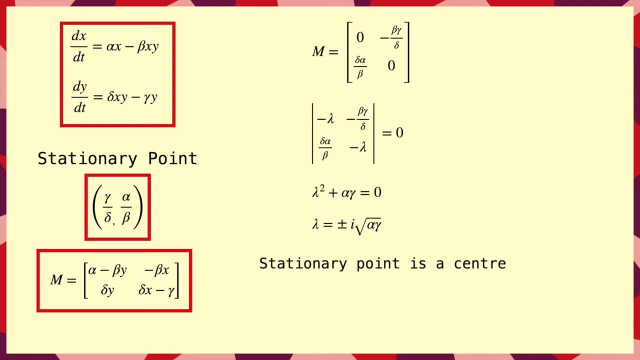 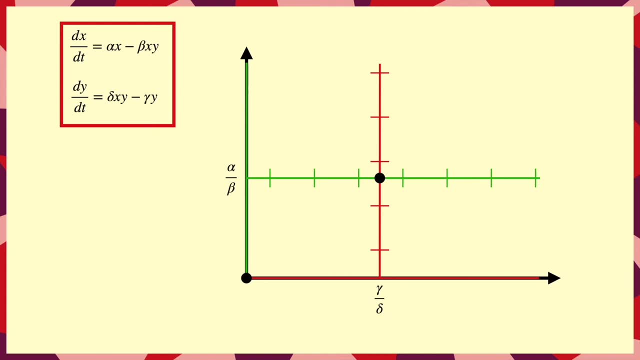 ellipses and just go round the fixed point. And now that we know about the fixed points we can draw our phase plane. Now the nullplanes split the plane into regions and we want to quickly check the direction that X and 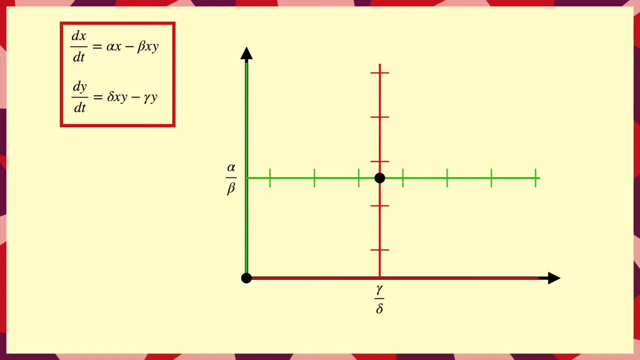 Y are moving in each region. This just helps us make sure that we draw the paths correctly. So we'll put a little arrow in each region to show whether X and Y are increasing or decreasing, And then finally we can draw some trajectories. 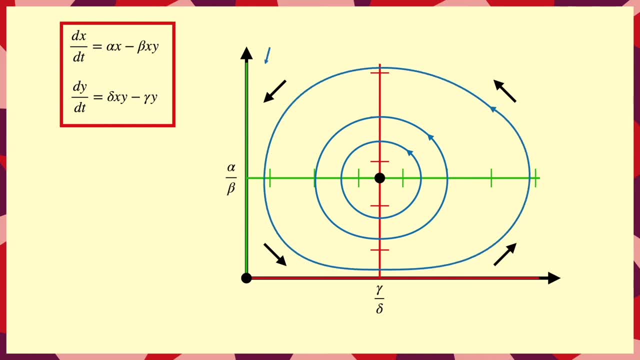 making sure that the two stationary points look like a saddle and a centre. Here I've drawn the trajectories as closed loops, but we don't know that that's actually correct. They could be slowly spiralling towards or away from the centre, But we can get a. 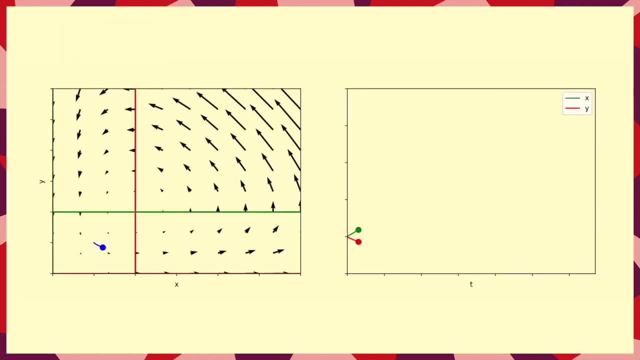 computer to draw the same thing for us Here. on the left we have the same plot. There's a vector field in the background showing the direction and speed of trajectories, And on the right is just a graph showing how X and Y evolve over time, And we can see. 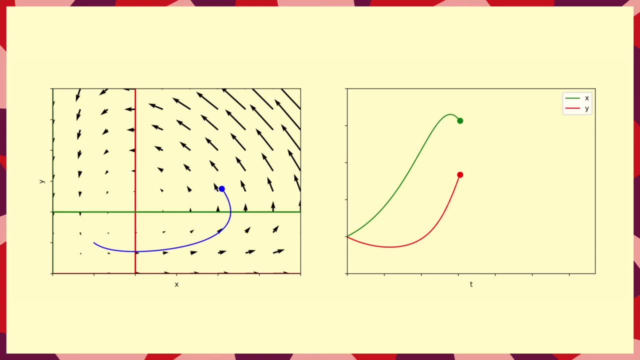 it looks periodic, with X, the prey population peaking first, followed by the predator population, And the trajectory does look like a closed loop. It lines up with itself each time it goes around. But can we prove why this is the case? 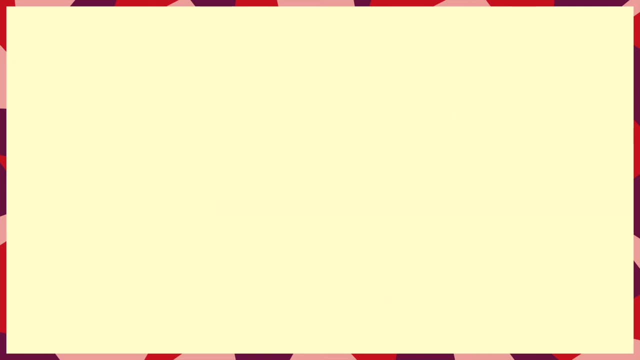 Well, if we want to do that, we need to look for a conserved quantity, a bit like energy in a physical system. So we need to find some combination of variables whose time derivative is zero. Well, to begin with, we can multiply our equations by delta and beta, so that the X, Y terms 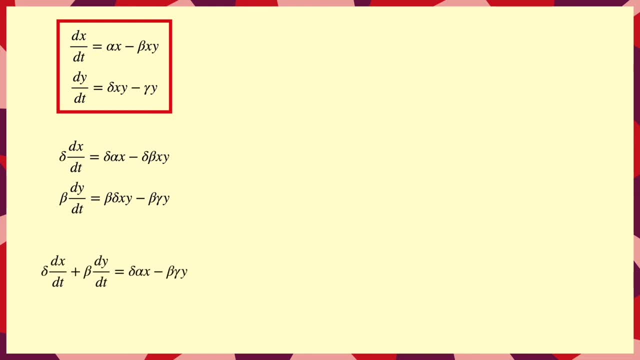 cancel out. But then we're left with some linear terms that we can't get rid of And the next step is a bit tricky if you don't know it. but we can actually look at what happens if you take the derivatives of log X and log Y.